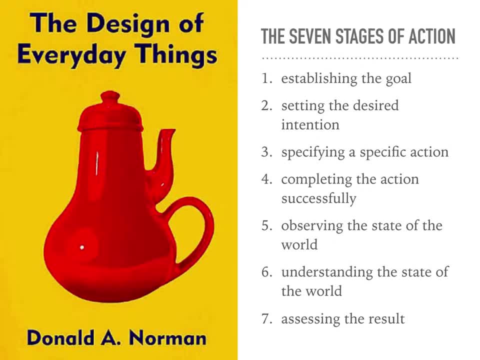 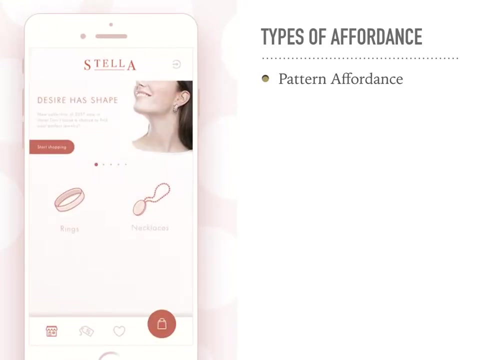 are as follows: Establish the goal, set the desired intention, specify a specific action, complete the action successfully. observe the state of the world, understand that state of the world and assess the results. A pattern affordance originates from previously learned behaviors and patterns. 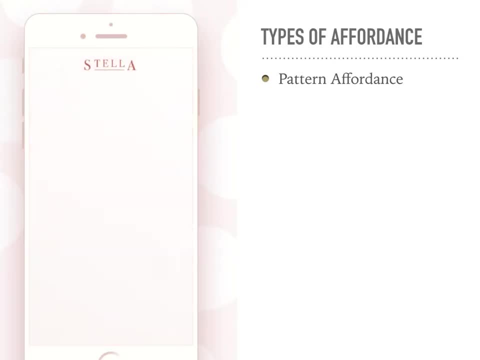 For instance, a clickable logo in a mobile experience is expected to take a user back to the home page. This is a pattern people have seen repeatedly, so users expect it. Text utilized in contrasting colors, perhaps underlined or italic, amid regular text. 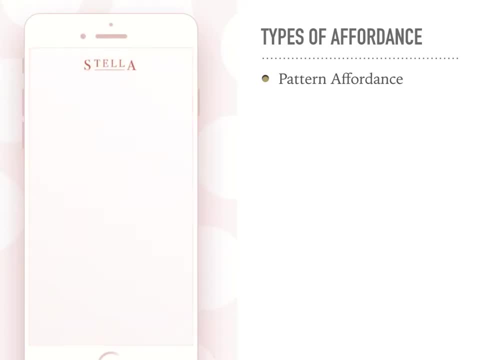 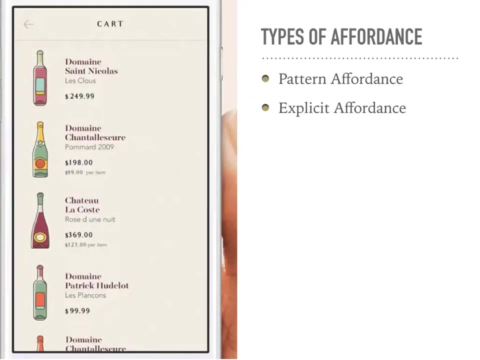 is expected to be a link. A graphic representation of a paper airplane has become so ingrained in our psyche that even the most inexperienced of users understands that it represents send Explicit affordance. All of the steps are noticeable because they deliver clear directions to the user. 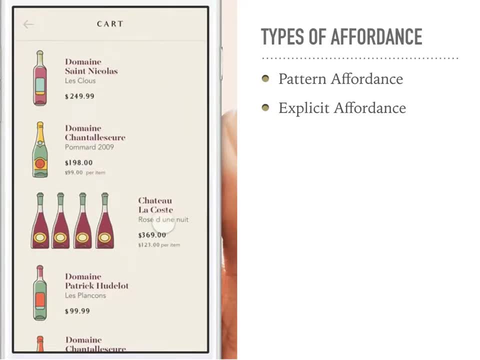 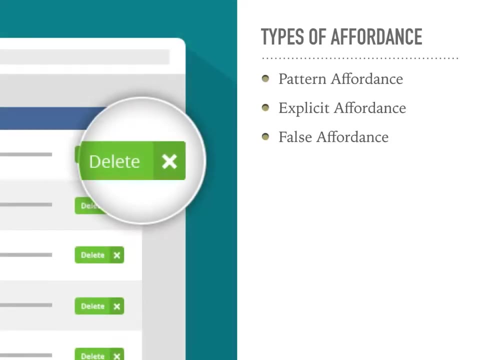 For example, a button with the words click here denotes a specific action or a form field which has placeholder text stating first name, last name. A false affordance customarily appears to afford an appropriate capability, but instead affords an unexpected one or none at all. 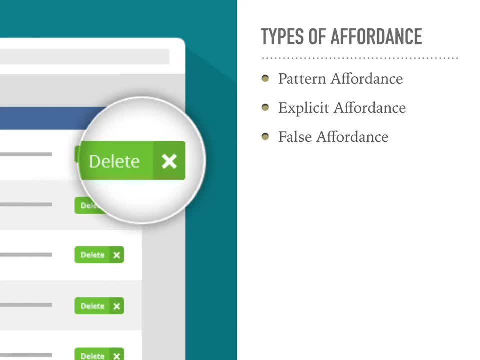 Some examples are: a non-interactive component might appear clickable due to a shadow or a button-like shape. The logo at the top of the page does not redirect the user to the home page as expected. An underlined sentence might appear to be a link. 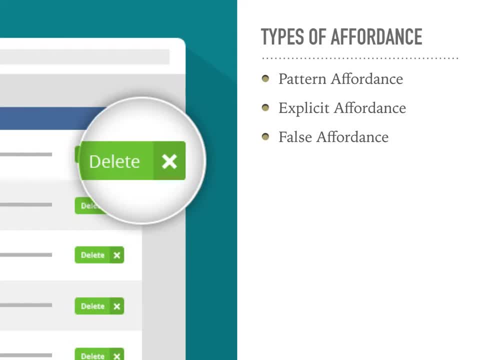 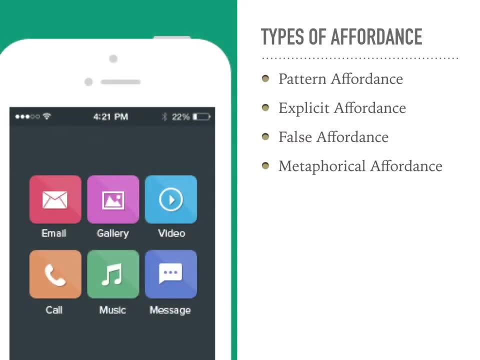 but instead it does nothing or, in this case, it adds more to the whole picture. Using the color green to denote delete Metaphorical Affordance, Things that graphically imitate real objects, to get across the idea of the design process. 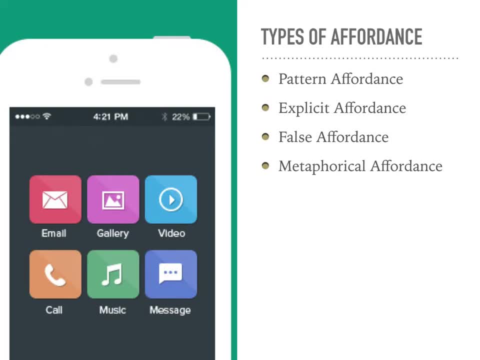 Iconography is a perfect example of metaphorical affordance when done well. Take the concept of delete: Its roots are in the metaphor of a physical trash can. Its icon is usually a trash bin. It is a beautiful example of a metaphorical affordance.